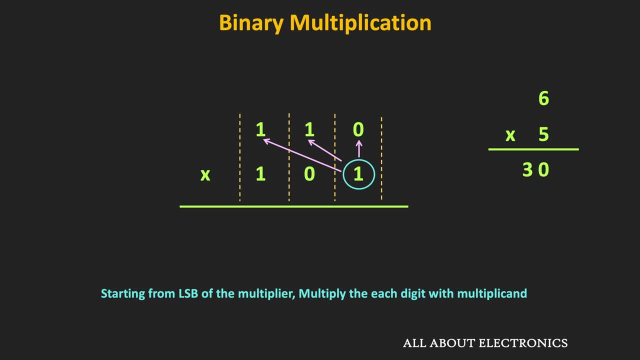 So there we have this행al variable. Now, when we are multiplying these binaryweults, then actually we are also multiplying their weights, And according to their weights we'll place the result in the particular column. So here, first, let us multiply this one with the zero. 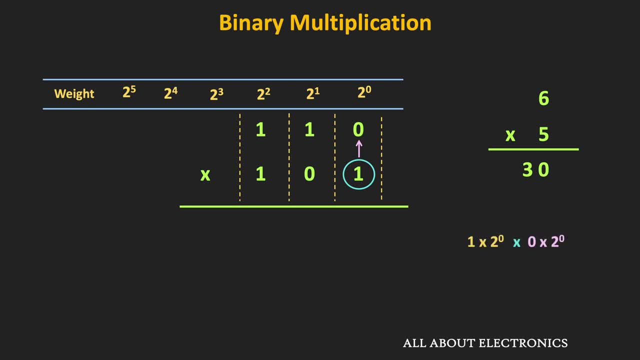 So here the weight of the both one and zero is equal to two times the zero, So the each digit will be equal to zero. So these aren't exact values here And, as you know, this 1 cross 0 is equal to 0.. 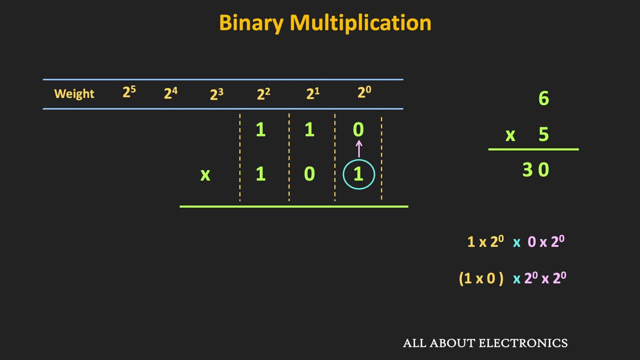 And if we multiply their weights, then it will be equal to 2 to the power 0. Therefore, we will place the result in this 2 to the power 0 column. Likewise, let us multiply this 1 with the 1.. 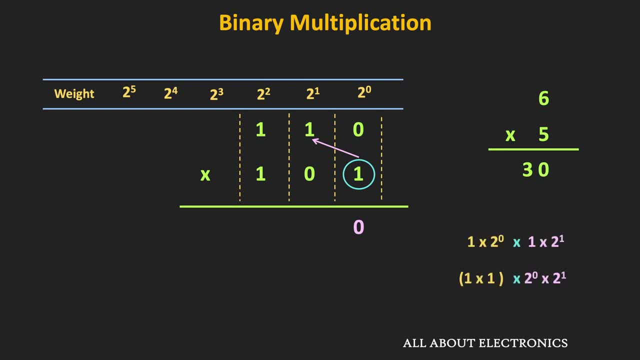 So here this 1 cross 1 is equal to 1. And if we multiply their weights then the result will be equal to 2 to the power 1.. Therefore, we will place the result in this 2 to the power 1 column. 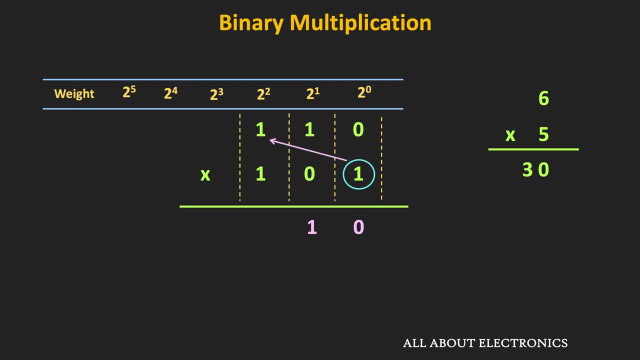 Likewise, let us also multiply this 1 with the MSB position. So once again this 1 cross 1 will be equal to 1.. And if we see their weights, then their weights are 2 to the power 0 and 2 to the power 2.. 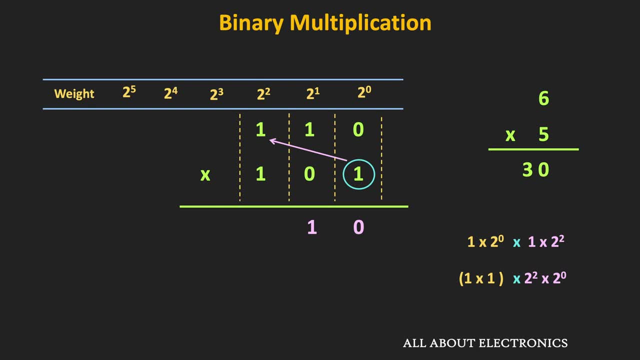 So if we multiply their weights then the result will be equal to 2 to the power 2.. Therefore we will place the result in this column. So in this way we have multiplied the first digit of the multiplier with the multiplicand. 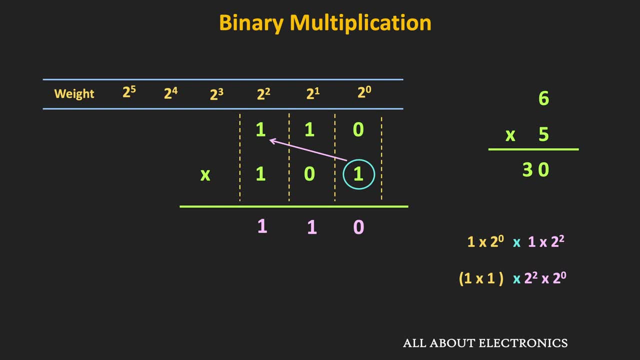 And in a way we got our first partial product. So, similarly, now let us multiply the second digit of the multiplier with the each digit of the multiplicand. So first let us multiply it with the 0.. So, as you know, this 0 cross 0 is equal to 0. 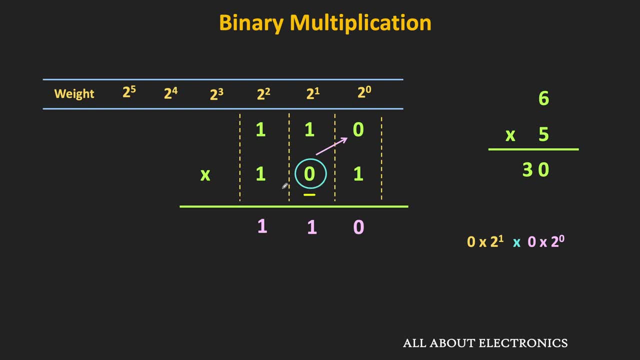 But here the weight of this 0 is equal to 2 to the power 1.. On the other hand, the weight of this 0 is equal to 2 to the power 2.. And if we multiply their weights, then their weights are 2 to the power 1.. 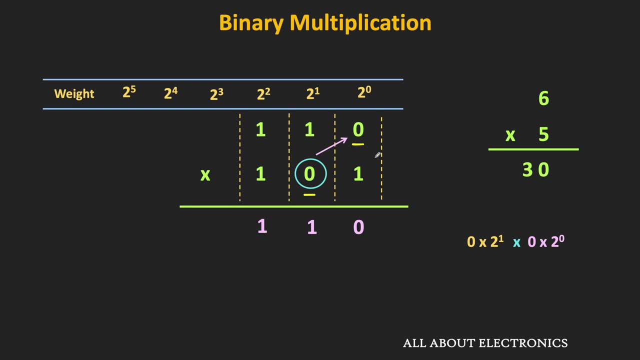 to the power 0. That means if we multiply their weights, then their multiplication will be equal to 2 to the power 1.. Therefore, we will place this 0 in this 2 to the power 1 column And, for our convenience, let us place the x over here. So, similarly, now let us 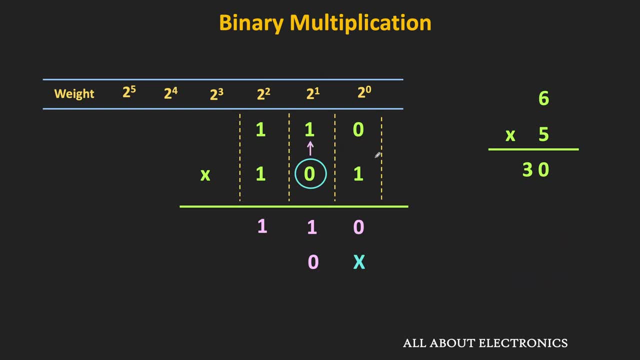 multiply this 0 with the 1.. So once again this 0 cross 1 will be equal to 0. And here if we see the weights of the both digits, then that is equal to 2 to the power 1.. Therefore, 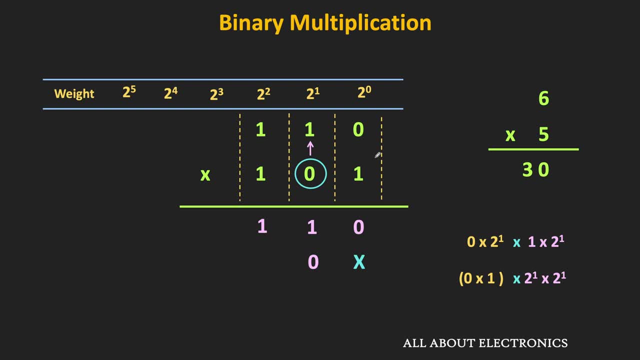 after the multiplication their weight will be equal to 2 to the power 2.. That means here we will place this 0 in this 2 to the power 2 column. And likewise now let us also multiply this 0 with the MSB. So once again this 0 cross 1 will be equal to 0. But now, if we 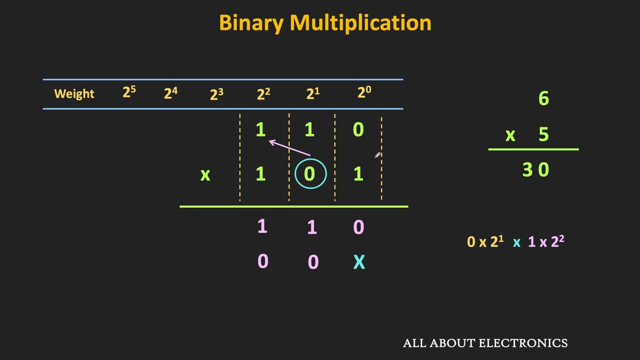 see their weights, then they are 2 to the power 1 and the 2 to the power 2.. Therefore their product will be equal to 2 to the power 3.. That means now we will place this 0 in. 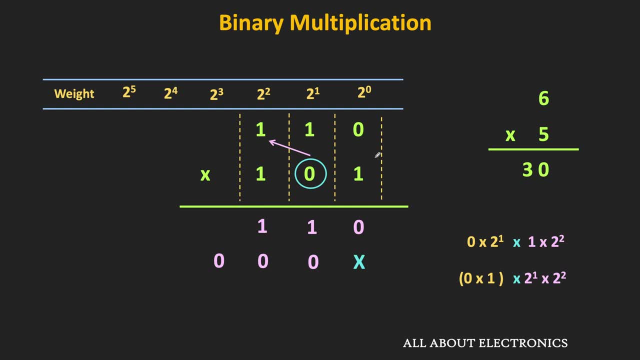 this 2 to the power 3 column. So in this way we got our second partial product. That means in a way we have multiplied the second digit of the multiplier with the multiplicand. So as you can see over here, while multiplying the second digit, this partial product is. 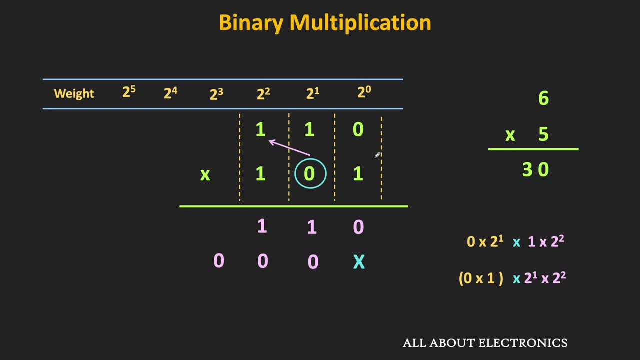 shifted to the left by a 1-bit position. So similarly, now let us move to the last digit and let us multiply it with the MSB. So similarly, now let us move to the last digit and let us multiply it with all the digits of the multiplicand. So first let us multiply this. 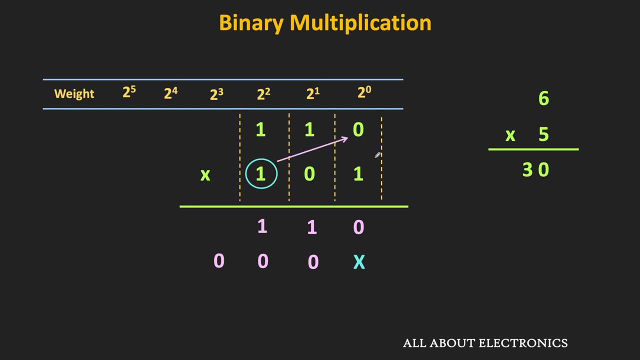 one with the 0. So once again this 1 cross 0 will be equal to 0.. And here if we see the weights of the two digits, then they are 2 to the power 2 and the 2 to the power 0.. 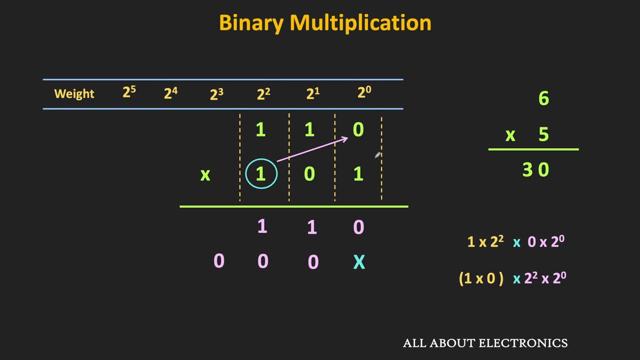 Therefore their product will be equal to 2 to the power 2.. That means now we will place this result in this 2 to the power 2 column, And for our convenience, let us mark cross over 2 to the power 2.. So here we have 2 to the power 2.. And for our convenience, 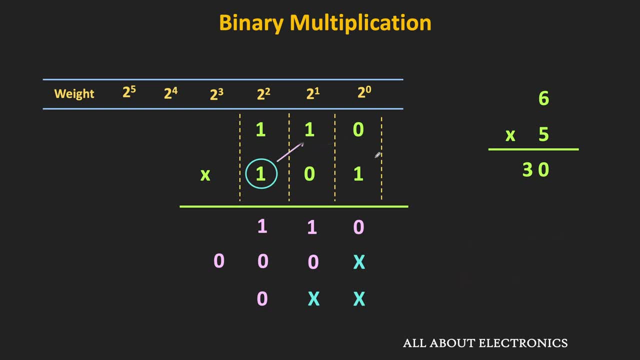 let us mark cross over 2 to the power 2.. And here we have 2 to the power 3.. So, similarly, this 1 cross 1 will be equal to 1. And this result will be placed in this 2 to the power. 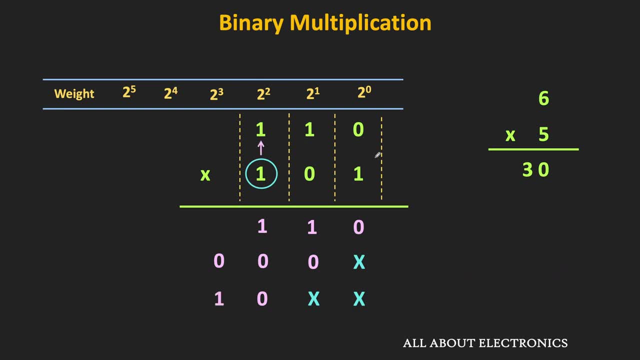 3 column. Likewise, this 1 cross 1 will be equal to 1.. And this product will be placed in the 2 to the power 4 column, Because here the weight of both digits is equal to 2 to the power 2.. So in this way we also got our third partial product. So as I said earlier, 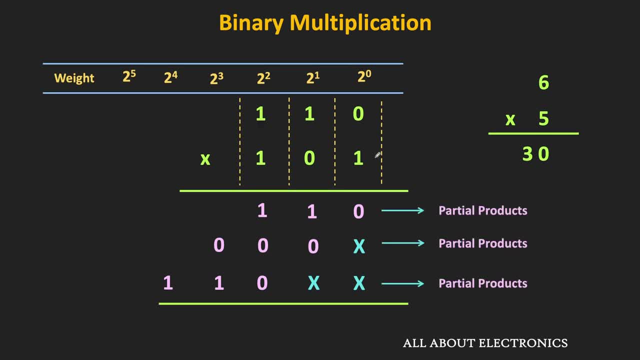 All these 3 are the partial products And if you see their value, then it is either 0 or their value is same as the multiplicand. So while multiplying, if the digit in the multiplier is equal to 1, then the partial 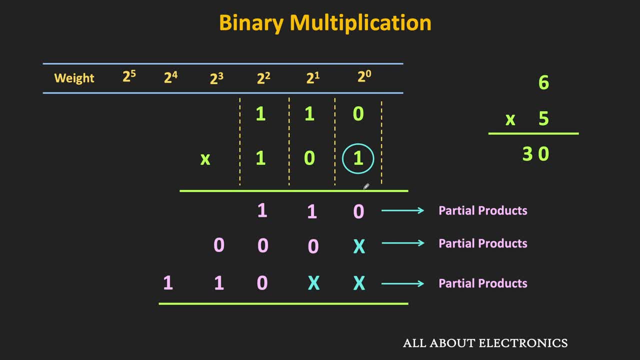 product will be same as the multiplicand, But if the digit is equal to 0, then the partial product will be equal to 0. So in this way the multiplication becomes much easier. And here, as we have seen, according to their weights, these partial products are left shifted. 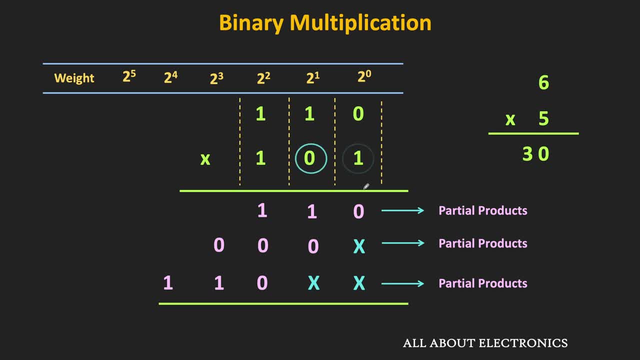 That means starting from the LSB of the multiplier. as we move towards the MSB, then each partial product will be left shifted by a 1-bit position And finally, once we get all the partial products, then we just need to add them to get the result. 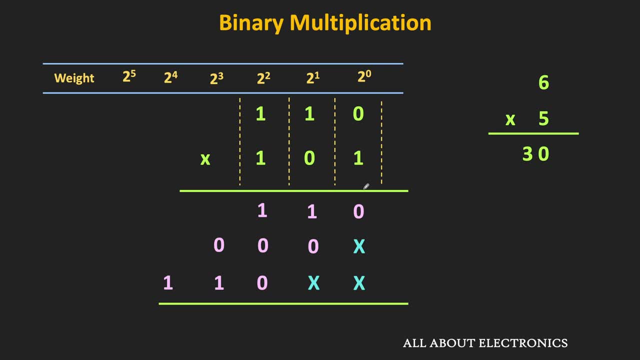 of the binary multiplication. So now, if we just do the column by column addition, then in the rightmost column we will have 0. Similarly, in the next column we will have this 1.. And likewise in the next 3 columns also, we will get the 1.. 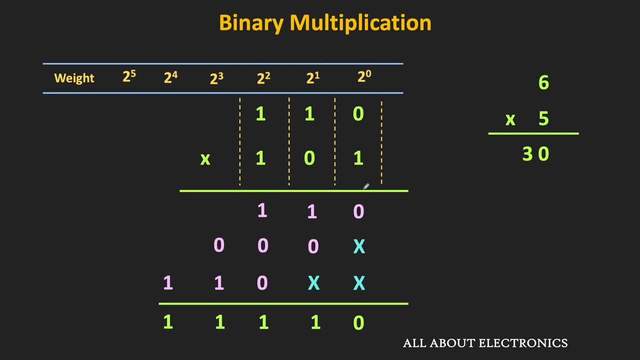 That means, after multiplying these two binary numbers, the product is equal to 11110.. And to cross-verify our result, let us convert it into the decimal, So it is equal to 16 plus 8 plus 4 plus 2.. 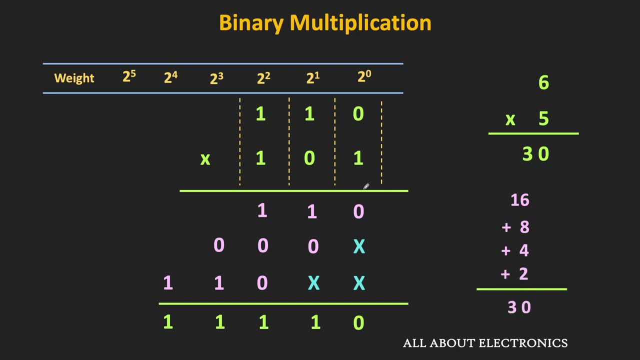 That is equal to 13.. That means indeed, our binary multiplication is correct, Thank you. So, as you have seen, in the binary multiplication we need to follow 3 steps. So first we need to multiply each digit of the multiplier to the multiplicand. 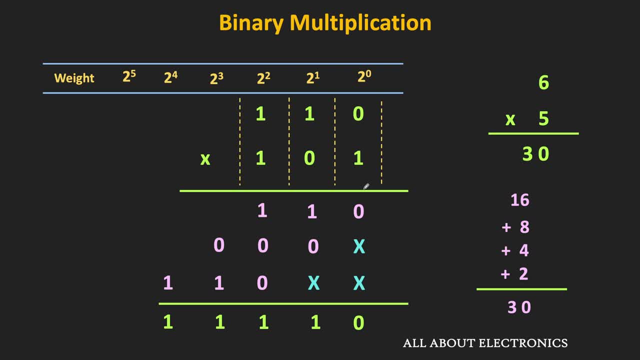 So if the digit of the multiplier is 0, then the partial product will be also equal to 0. But if the digit is equal to 1, then the partial product will be same as the multiplicand. So in this case, as you can see, whenever the digit of the multiplier is equal to 1,. 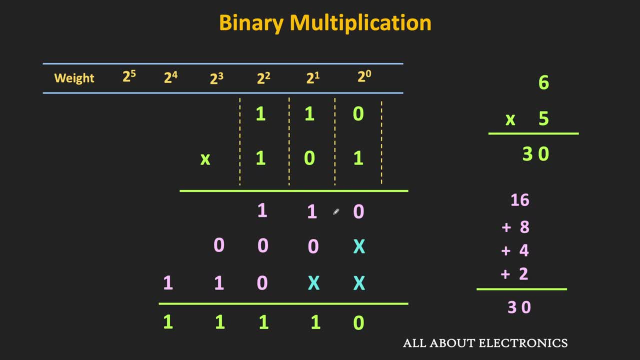 then the partial product is same as the multiplicand, That is, equal to 1110.. Also, while multiplying the each digit of the multiplier to the multiplicand, as we move from the LSB towards the MSB, then the each partial product is also left shifted. 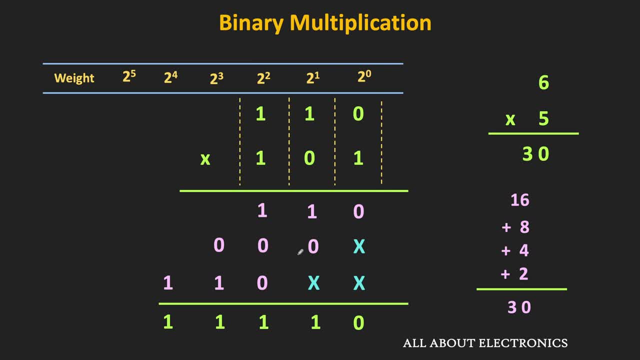 by a one-width position And then, once we get all these partial products, then we just need to add them to get the final result. So let us take one more example so that it will get clear to you. So let's say, we want to multiply this 12 and the 13.. So, in the decimal, we need to multiply this 12 and the 13.. So, in the decimal, we need to multiply this 12 and the 13. So, in the decimal, we need to multiply this 12 and the 13.. 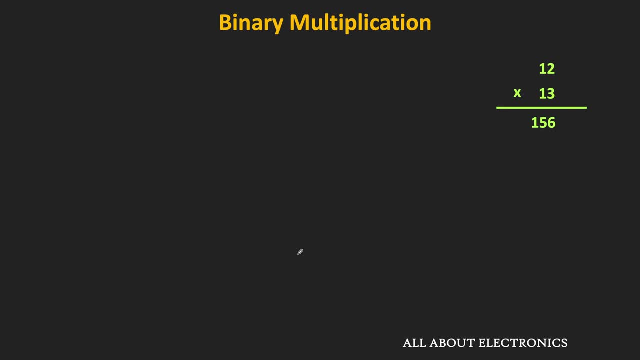 So in the decimal this result should be equal to 156.. So let us see the same thing in the binary multiplication. So in the binary this 12 corresponds to 1100 and similarly this 13 corresponds to 1101.. 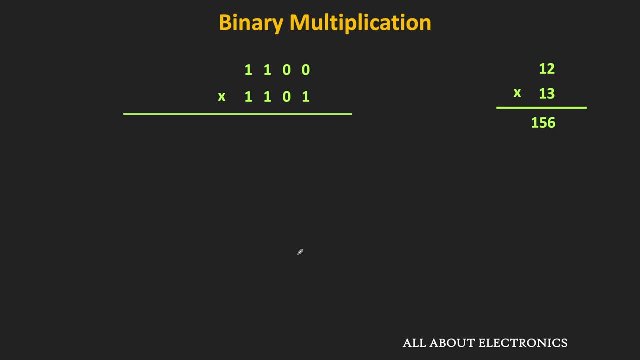 So first let us start with the LSB of the multiplier. So in this case that is equal to 1.. So since this digit is equal to 1, so the partial product will be same as the multiplicand. So in this case that is equal to 1100. 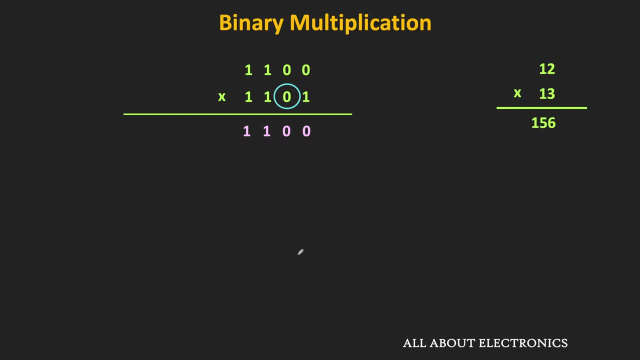 So then after if we move to the next bit, then that is equal to 0. And since it is 0, so the partial product will be also equal to 0. But now it will be left shifted by a one-bit position. 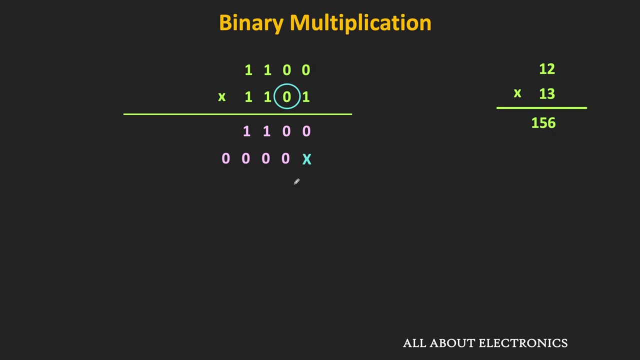 So in this position let us mark x, So after that, if we move to the next bit, then that is equal to 1.. So, since it is 1, so the next partial product will be same as the multiplicand. So in this case that is equal to 1100. 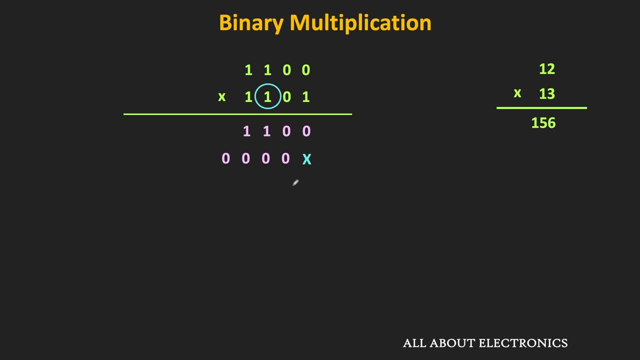 So in this case that is equal to 1100.. multiplicand That is equal to 1100.. But now, once again, it will be left shifted by a one mid position. Therefore, these two positions have been crossed. And finally, if we see, 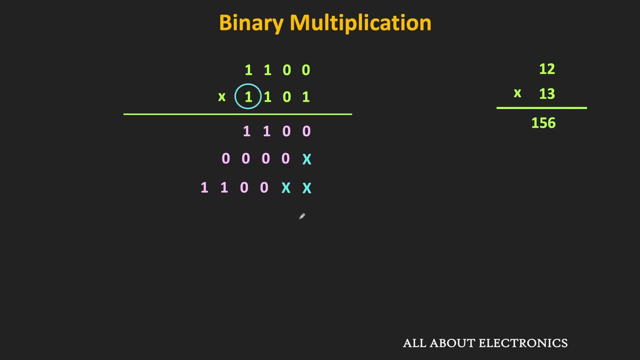 the MSB of the multiplier, then that is equal to 1.. So once again the partial product will be same as the multiplicand, But once again it will be left shifted by a one mid position. So in this way we got our all the partial products. So the next step is the addition. 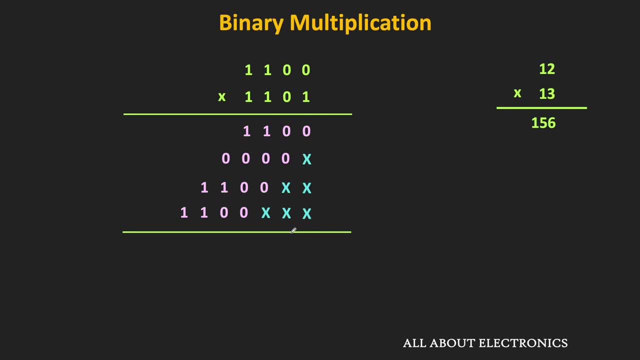 of all these products. So once again we will do the column by column: addition. So in the rightmost column we will have 0. And if we move to the next column then once again the result will be equal to 0. Then after, if we move to the next column, then the result: 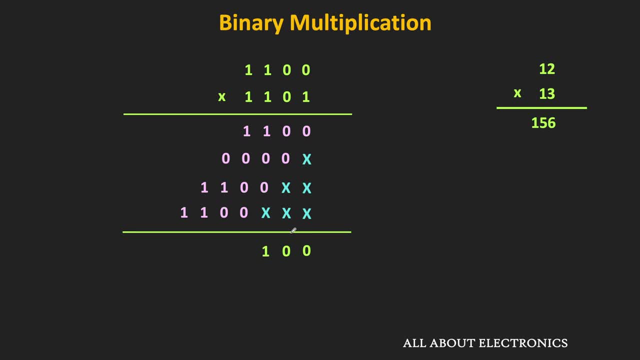 will be equal to 1.. And then after, in the next two columns also, the result will be equal to 1.. Then, after this, 1 plus 1 will be equal to 0 and the 1 will be the carry. 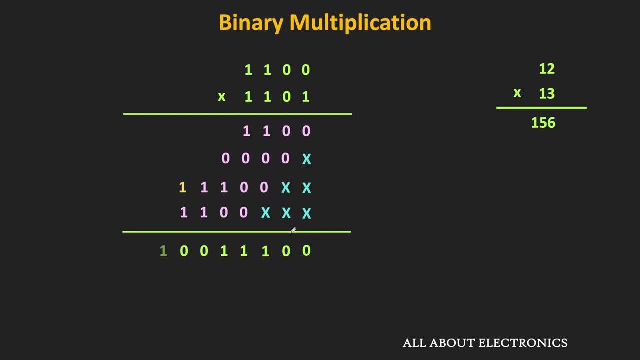 And once again this 1 plus 1 is equal to 10.. So this is the result after the multiplication. And to verify the result once again, let us convert it into the decimal equivalent. So in the decimal this digit corresponds to 128 plus 16 plus 8 plus 4.. 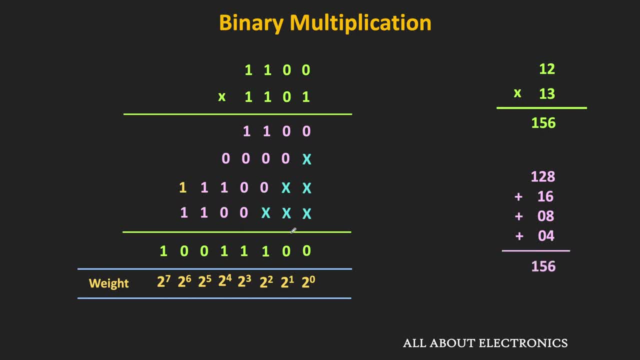 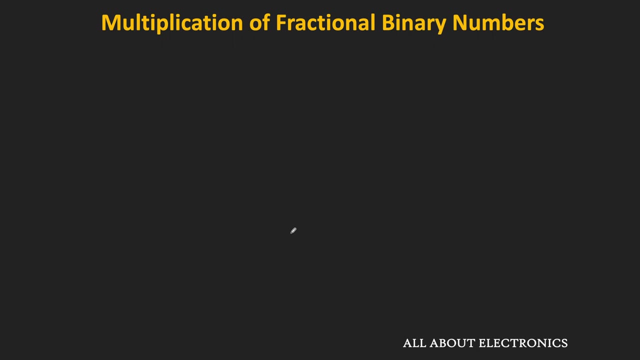 And that is equal to 156.. And therefore, this is the result after the multiplication. So in this way we can multiply two binary numbers. So similarly, now let us see how to multiply the fractional binary numbers. So the multiplication process for the fractional binary numbers is also very similar to the 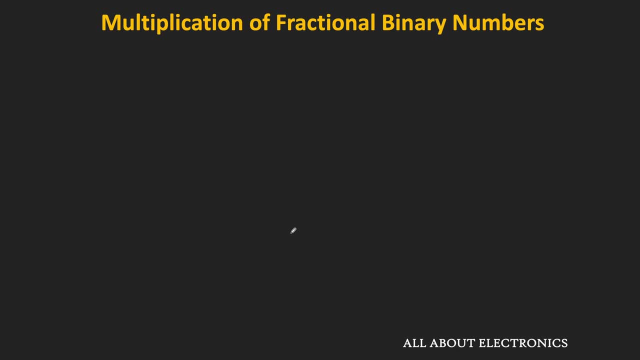 binary integers. So let us take one example and through that let us understand the multiplication process. So let us say we want to multiply these two fractional numbers, So if we see the decimal equivalent, then that is equal to 6.25 and 3.5.. 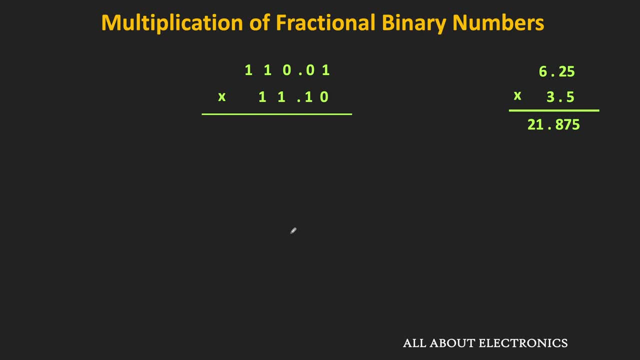 And the result after the multiplication will be equal to 21.875.. So now let us see how to perform that multiplication in the binary. So if you see the first number, then in this number the number of digits in the fractional part is equal to 2.. 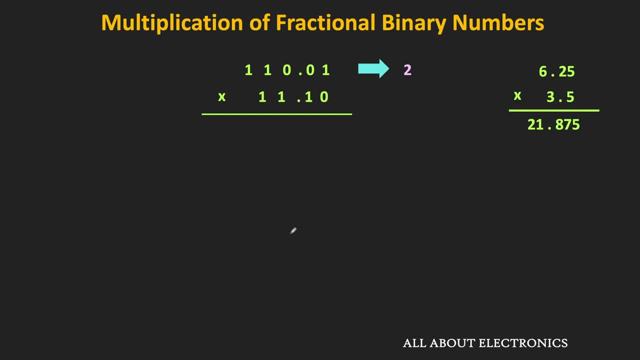 Similarly in the second number the number of digits in the fractional part is equal to 1. Because here this zero does not carry any weight, And even if we put three zeros after that, then also the value of the number will remain. 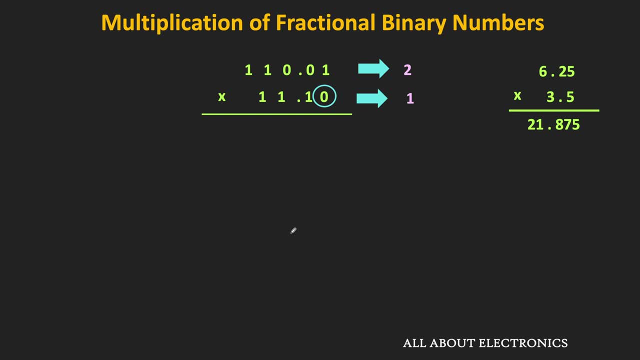 same. So just keep this thing in the mind And for a moment, for this binary multiplication, just ignore these binary points. So here to perform the binary multiplication. these two numbers are written after removing their binary points. So now we will do our usual multiplication. 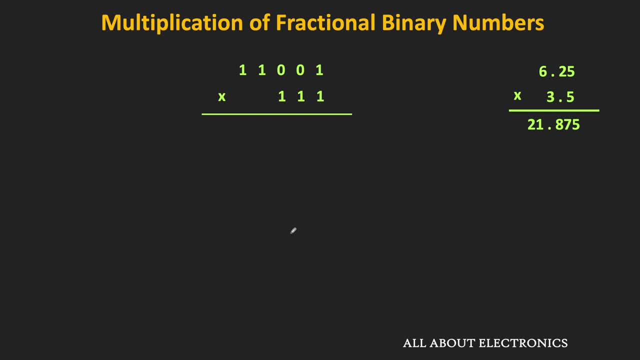 And once we get the final result, then we will place the binary point based on the number of fractional digits in each number. But first let us multiply these two numbers. So, starting from the LSB of the multiplier, the first digit is equal to 1.. 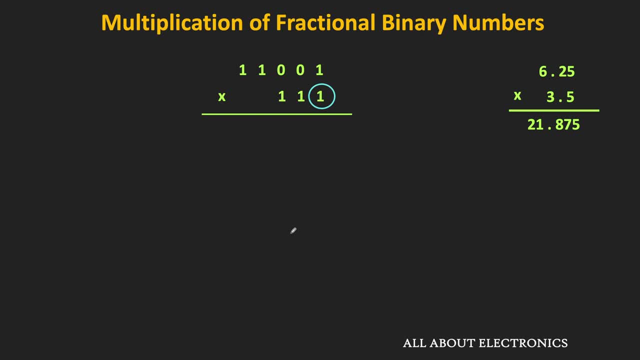 Therefore, the first partial product will be same as the multiplicand, That is equal to 11001.. So now, if we move to the next bit, then that is equal to 1.. So once again, the next partial product will be same as the multiplicand. 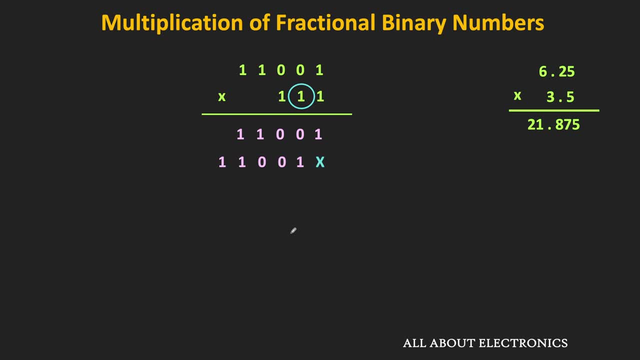 But now it will get left, shifted by a 1-bit position And after that if we move towards the MSB, then that is equal to 1. So once again the next partial product will be same as the multiplicand. 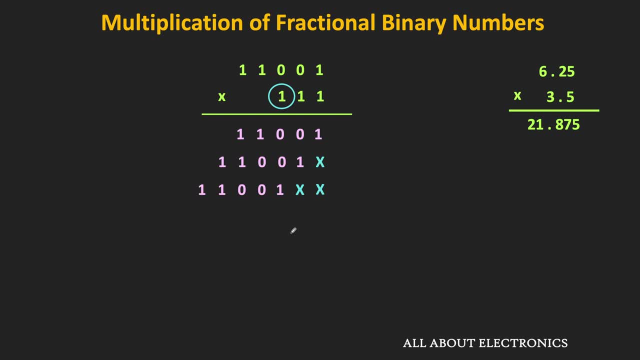 But once again it will get left, shifted by a 1-bit position. So in this way we got our all the partial products. So now if we perform the addition of all the partial products, then we will get the 1.. 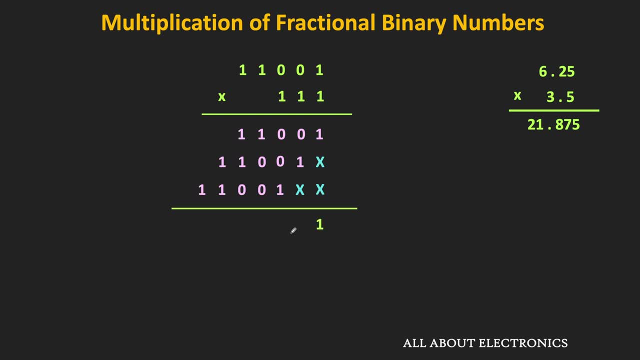 Then in the rightmost column we will get 1.. Then after, if we move to the next column, then that is also equal to 1.. And after that in the next two columns also we will get 1.. So then after in the next column, this 1 plus 1 is equal to 0 and 1 will be the carry. 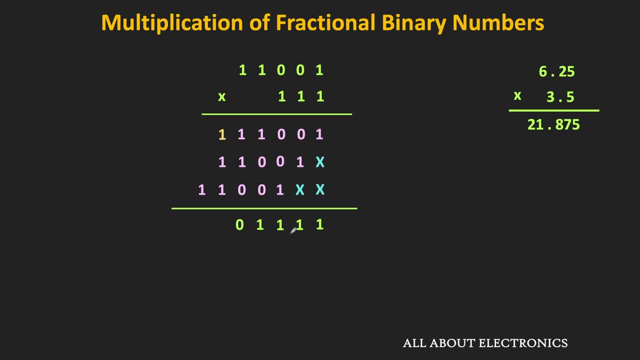 to the next column. So now in the next column, this 1 plus 1 plus 1 is equal to 1, and there will be a carry of 1 in the next column And once again this 1 plus 1 is equal to 1, 0.. 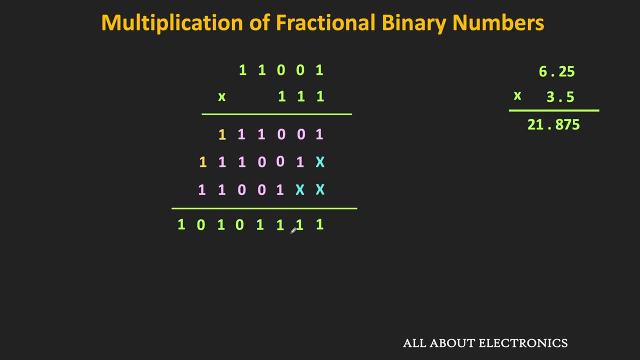 So in this way we got our result after the multiplication. So now we just need to put the binary point at the appropriate location. So, as we have seen in the first number, the number of bits after the binary point is equal to 2.. 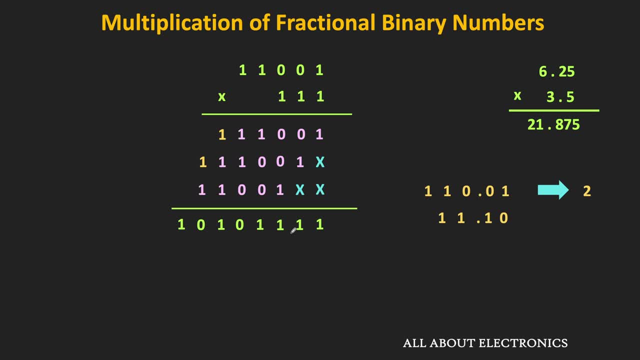 Likewise, in the second number, the number of digits after the binary point is equal to 1.. And this 2 plus 1 is equal to 3.. So in the final result, So in the final result, We will put the binary point after the 3 digits from the LSB. 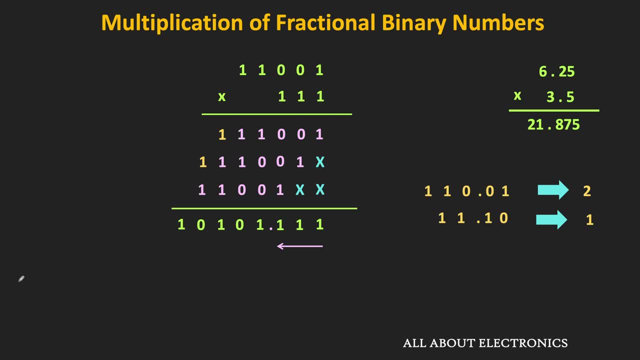 That means this is the result after the multiplication. But let us also verify our result by converting this binary number into the decimal equivalent. So if we see the decimal equivalent number, then that is equal to this: 16 plus 4 plus 1 plus 0.5 plus 0.25 plus 0.125. 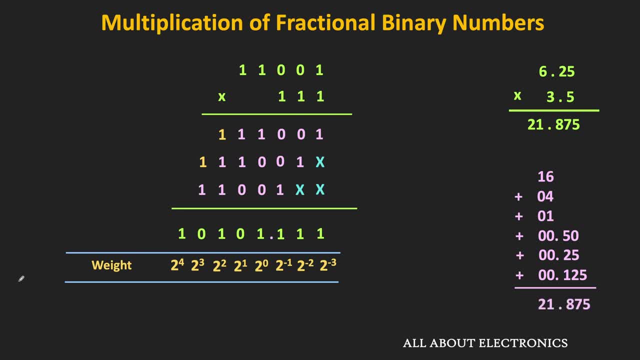 And that is equal to 21.87.. That means this is the result after the multiplication. So in this way we can also multiply the two fractional binary numbers. So let us take one more example so that it will get clear to you. 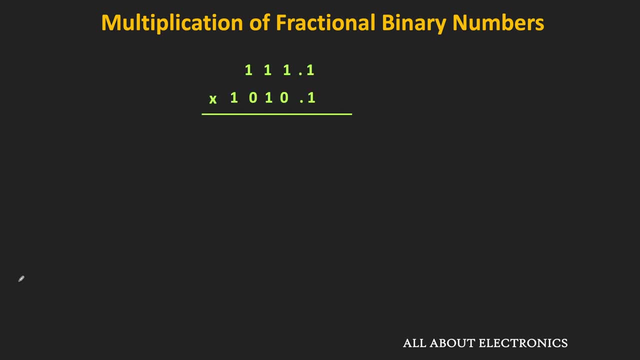 So let's say we want to multiply these two numbers. So if we see the decimal equivalent of the two numbers, then that is equal to 7.5 and the 10.5.. And the product of these two numbers will be equal to 78.75.. 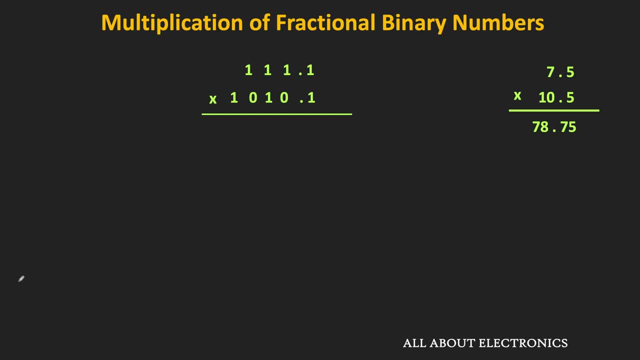 So if we see the decimal equivalent of the two numbers, then that is equal to 7.5 and the 10.5.. So let us see how to multiply them in the binary. So in both the numbers the number of digits after the binary point is equal to 1.. 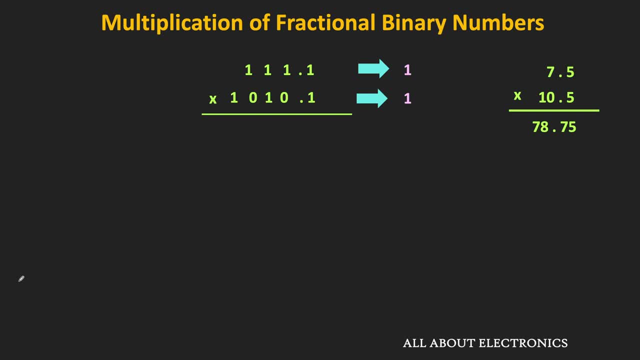 So for our time being, let us ignore these binary points and let us multiply these two numbers as the normal binary numbers. So here, starting from the LSB of the multiplier, if we see the first digit, then that is equal to 1.. 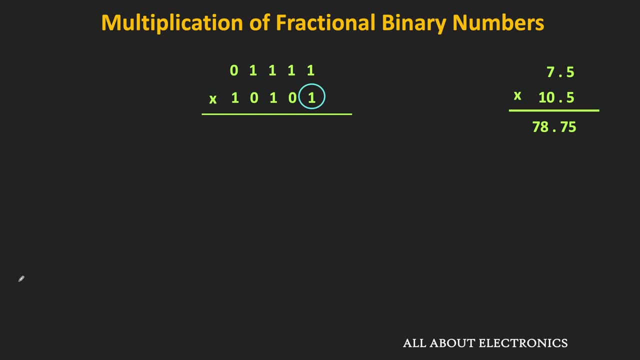 So if we multiply it with the multiplicand, then the result will be same as the multiplicand. So if we multiply it with the multiplicand, then the result will be same as the multiplicand. So if you pull down the value of a value, then replace the second result. 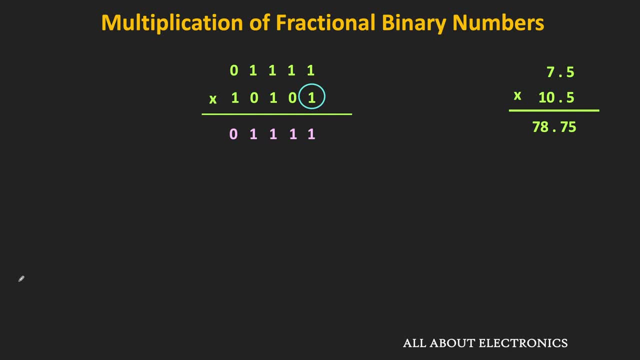 So let us simple multiply it with the last digit. So let us understandable check that the first digit is equal to 1.. So let us, Breatszyst, denominate this as revelation. So of course, at this right moment, the sum will be산 to be 0 too. 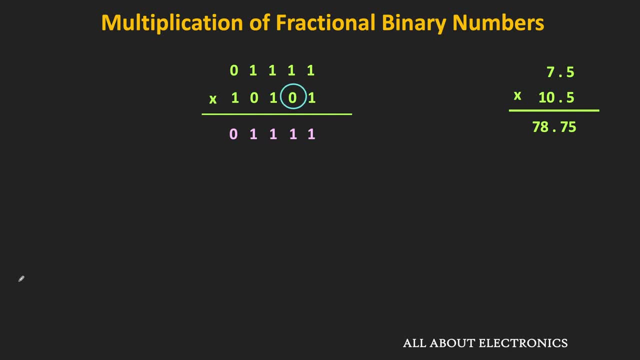 That is equal to 0x01111 and similarly, if we move to the next digit, then it is equal to 0. Therefore, we have been given the sum of the knitting items, and then we will be given 0x01111fferщil landscapes. 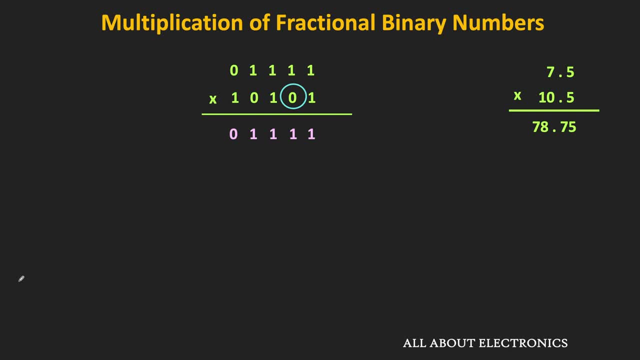 So the second partial product will be equal to 0. But now it will be left shifted by a one-bit position as a multiplication value. Then after, if we move to the next bit, then that is equal to 1.. So once again the partial product will be same as the multiplicand.